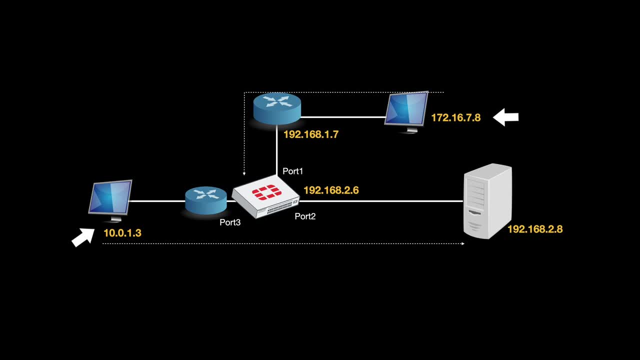 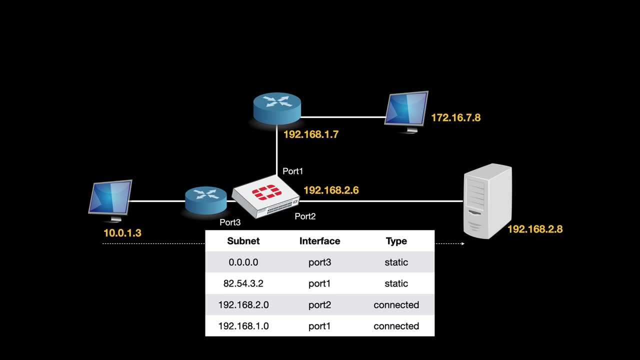 then the packet will drop. The reason is as following: If we look at the routing table, then everything becomes much more clear. So in our FortiGate routing table we can see that port 3 has a default route. It is quad zero, So our client can get out and reach its destination, since we have a route to the source IP. 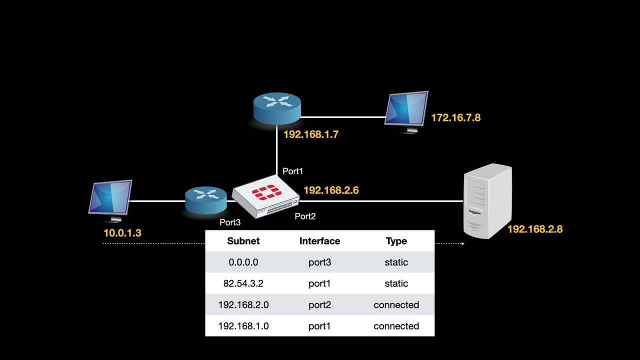 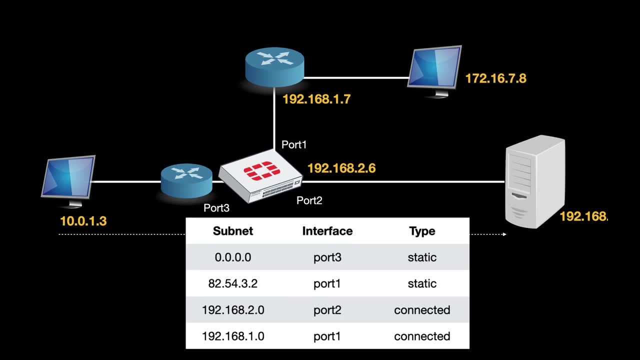 Now the other client, Now the other client, Now the other client. The 172.16 goes out through port 1.. In port 1,, if we look at the routing table, we have a static route to a network or to a destination at the 8254.. 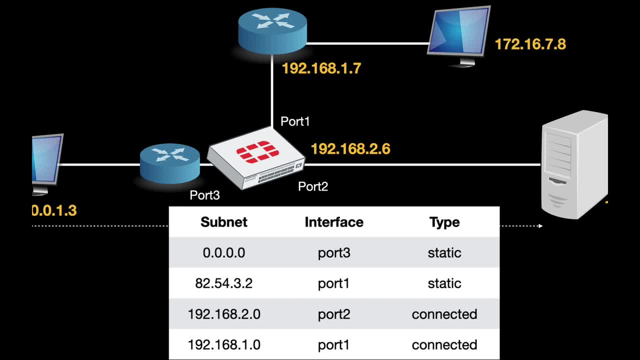 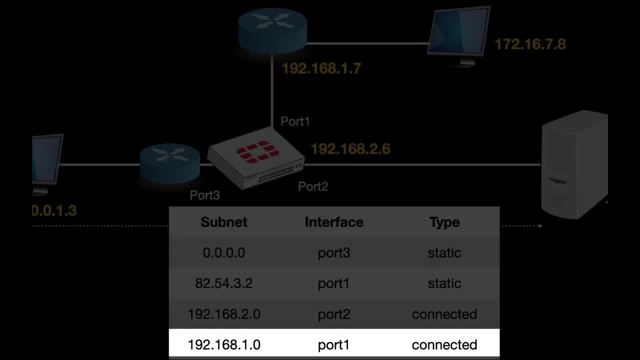 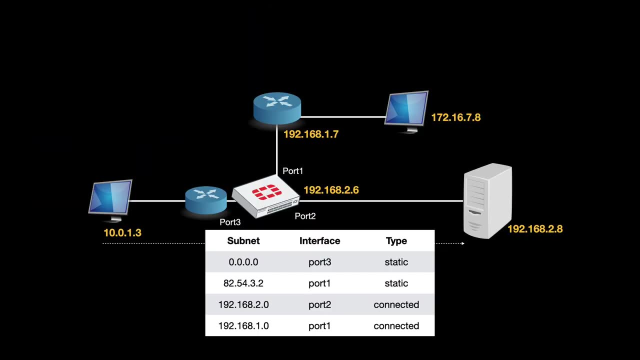 That is not our destination And we have another connected network which is the 192.168.1.0.. So port 1 doesn't have a route back to our 1.. The 172.16 and the packet is dropped. 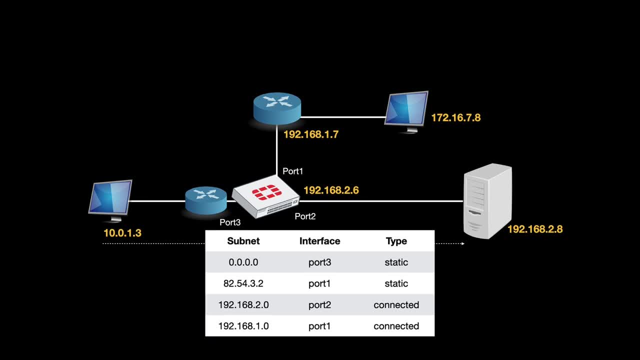 Now there are two types of RPF. There is the strict RPF and there is the loose RPF. The loose RPF tells us that there needs to be a route to the source IP. The strict RPF tells us that we need to have the best route to the source IP. 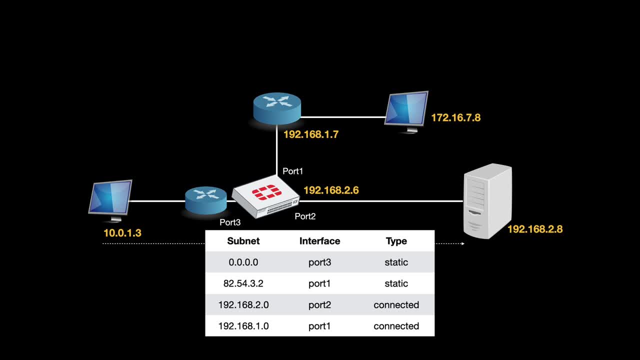 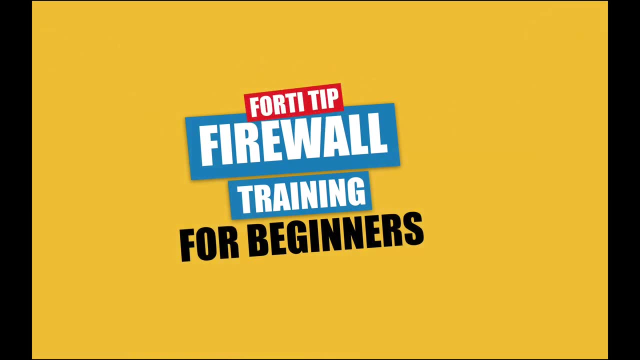 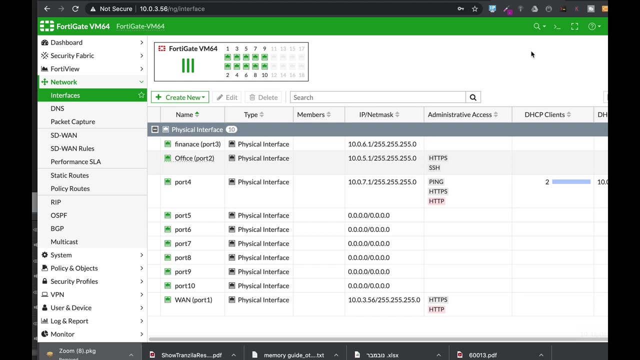 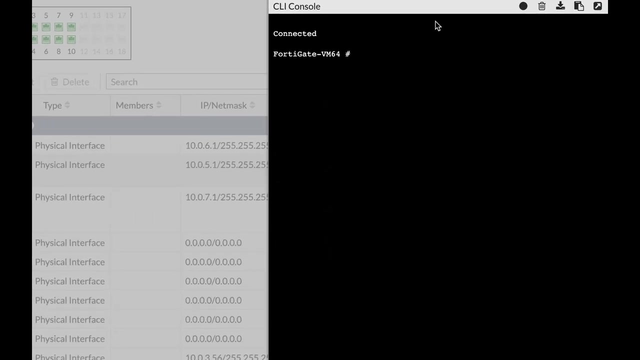 It can be configured on your firewall. Let's see how. All right, So that was a long opening, but it is important to understand how RPF actually works. So to configure RPF either in a strict mode or a loose mode you actually use. 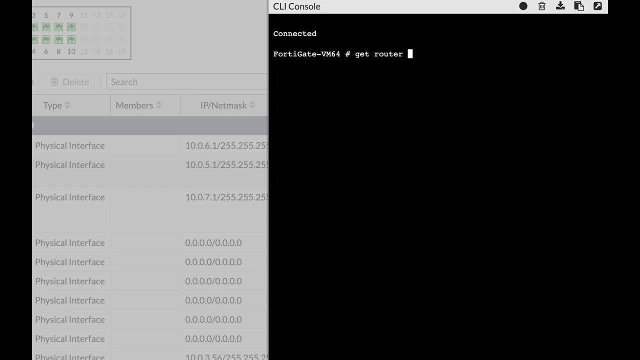 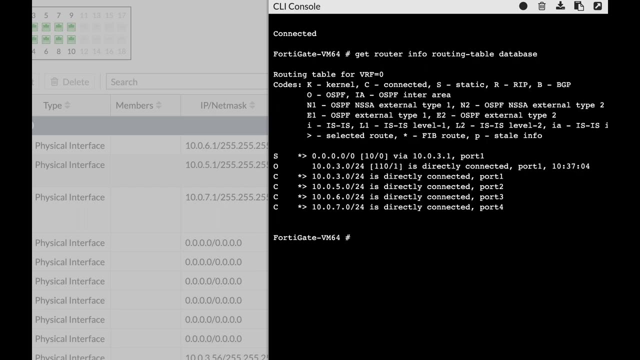 You know what? Let's just look at our routing table: Router info, Router info- Let's use the database, All right, So that's our routing table. We have an OSPF route, We have connected networks and we have a static route, which is the default route.